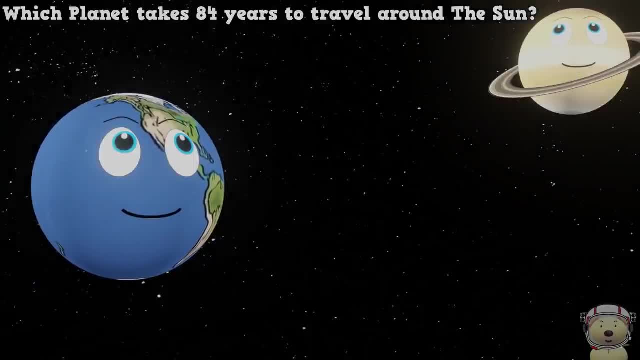 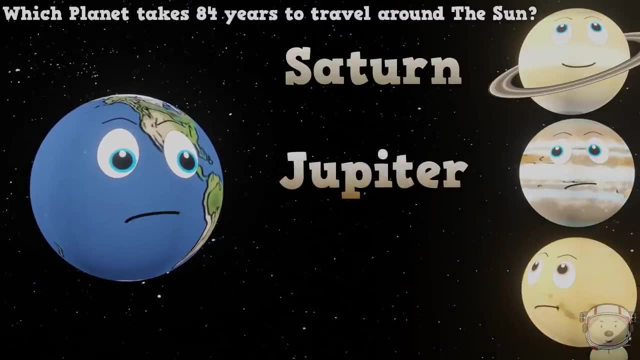 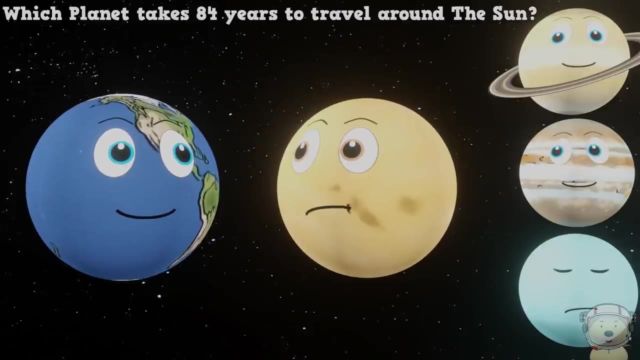 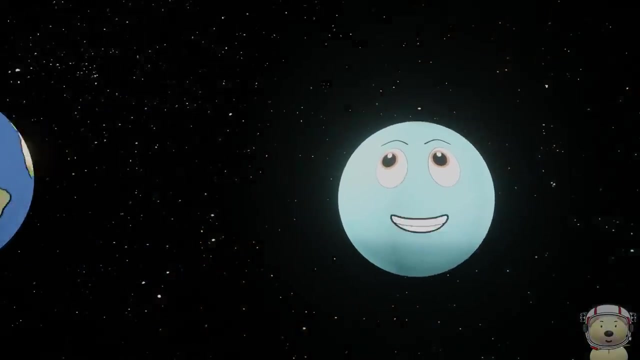 A- Saturn, Hey dudes. B- Jupiter, Hello. C- Uranus, Venus, not you. C is planet Uranus. What Not me again? Sorry, I'm watching you. Yes, it's me, planet Uranus. 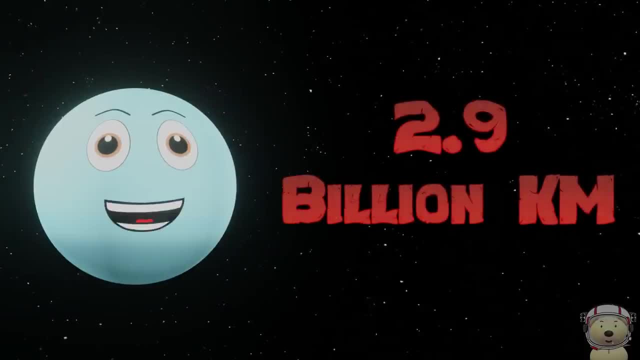 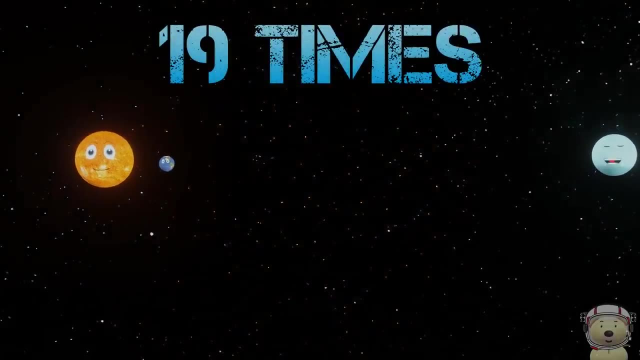 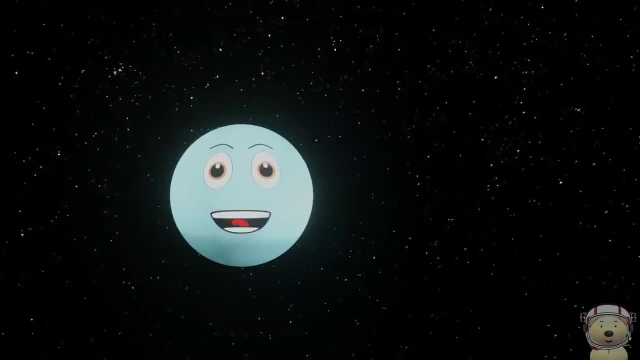 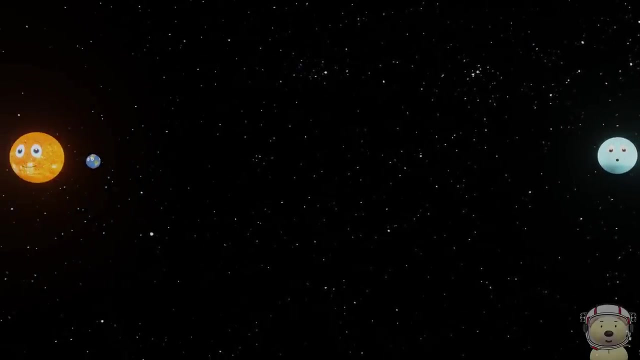 I am an average 2.9 billion kilometers from the Sun. That is, 19 times further out than the Earth. That means I am so far from the Sun. That means I am so far from the Sun that it takes me 84 years to orbit. that is a very long time. 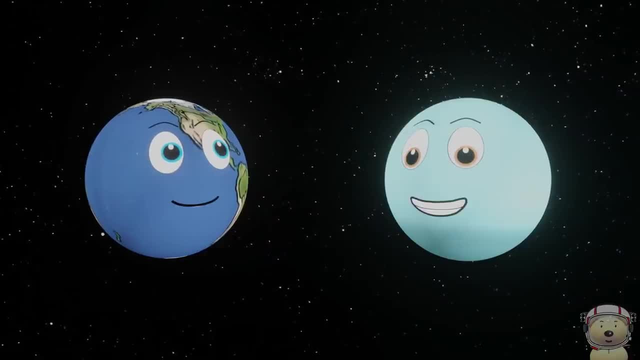 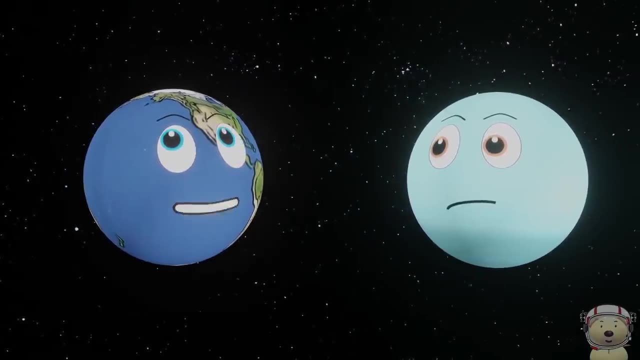 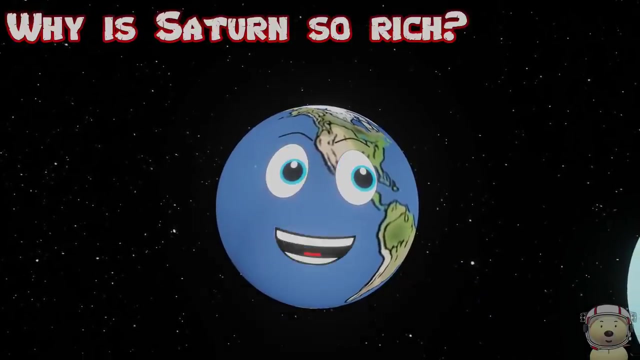 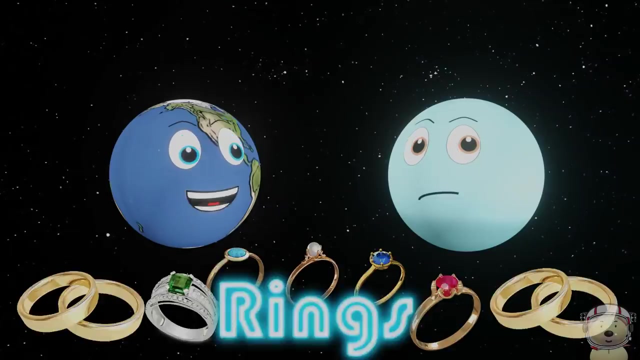 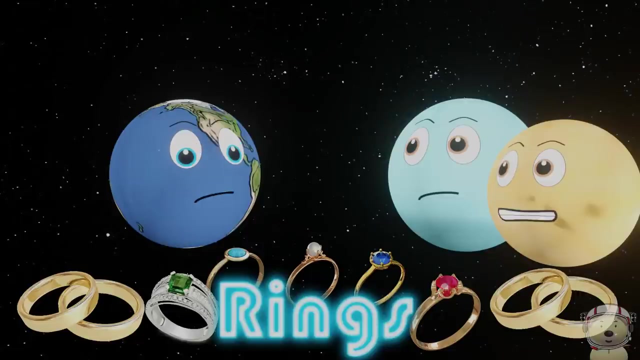 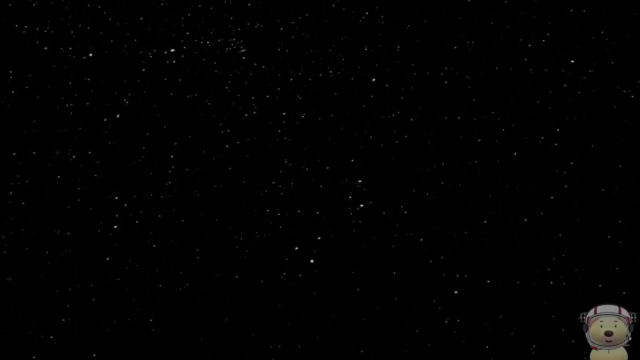 is that why you're grumpy, grumpy me. what are you talking about? hey, uranus, i've got a space joke for you. oh great, why is saturn so rich? i don't know, because it has lots of rings. i'm doing the next quiz: what is the brightest planet in the night sky? 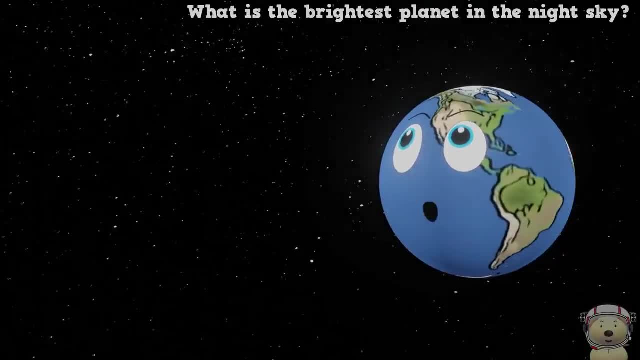 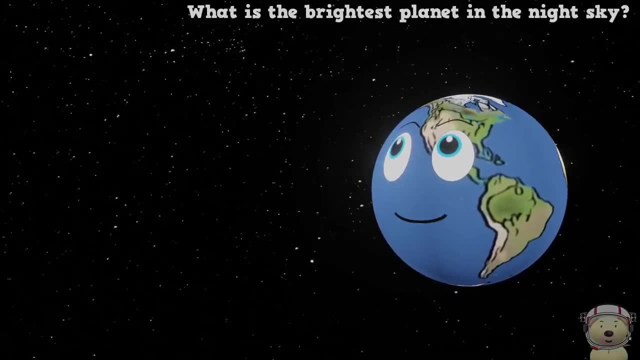 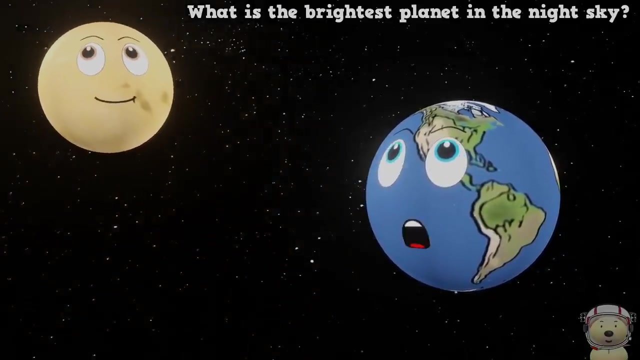 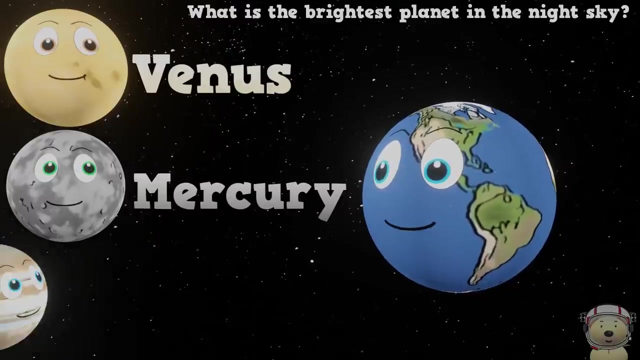 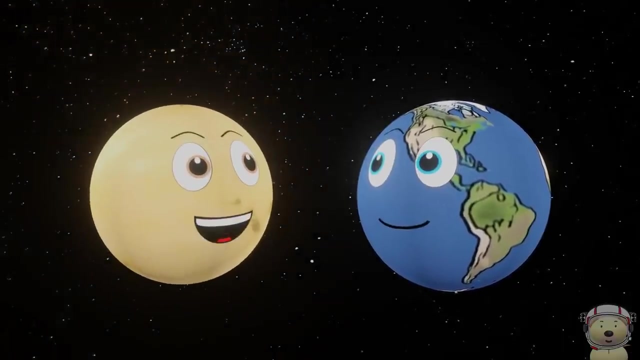 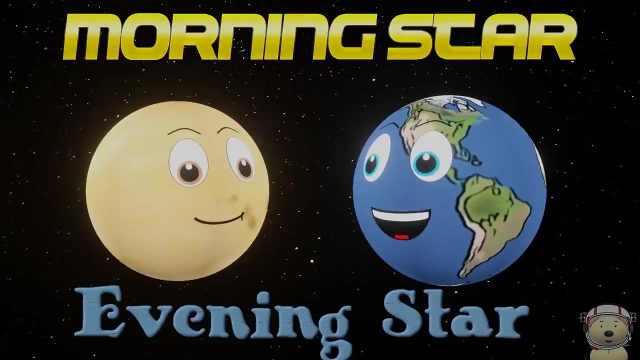 a venus, venus, the venus. you've got to be kidding me. after all the moaning, she's done. venus, you're on, okay, okay, no need to shout. b, mercury, hey, hey, c, jupiter, what's up? and the answer is venus. venus is also known as morning star and evening star. 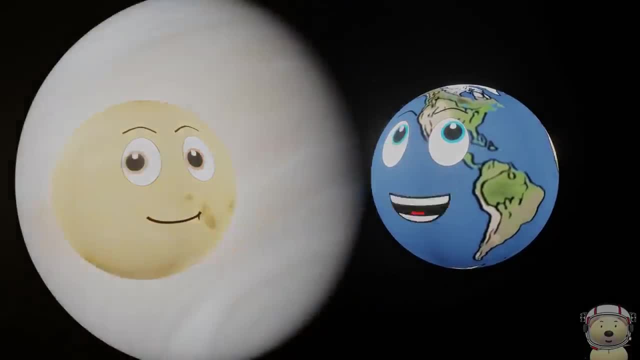 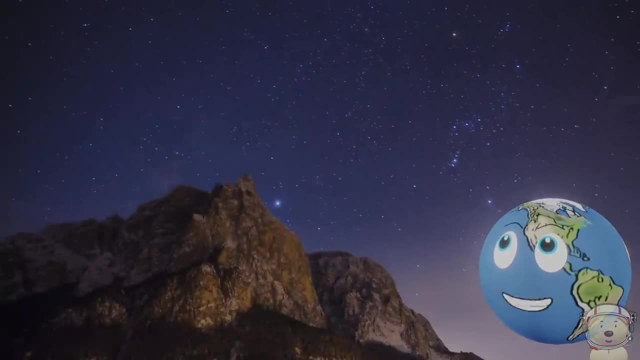 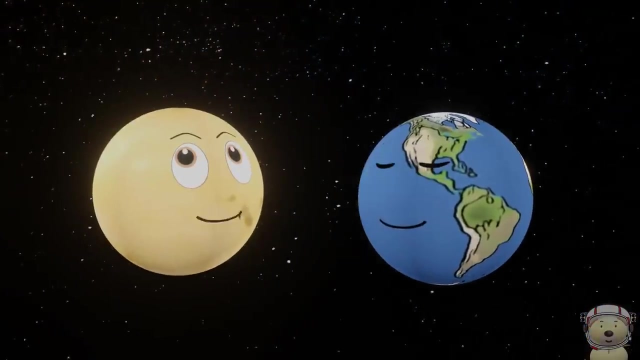 because the planet is so bright. it is so bright because it is covered by clouds that reflect much of the sunlight. it is actually the third brightest object in the sky, after the sun and the moon, so that means i'm the brightest planet in the solar system. what well bright.